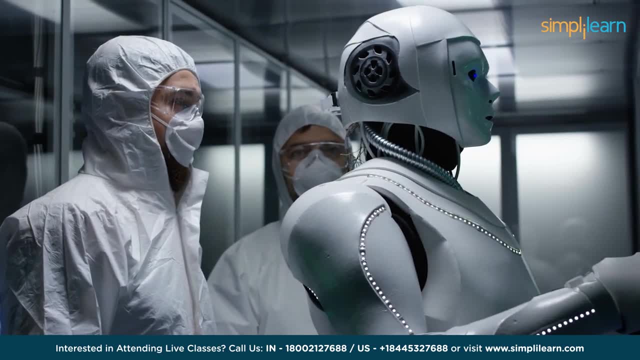 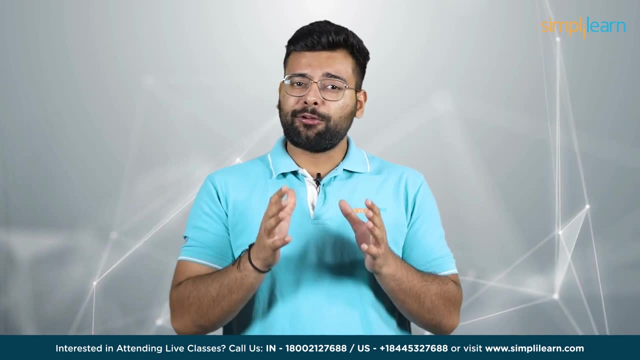 They yearned to push the boundaries of what was possible, to create mechanical beings capable of emulating human tasks. It was a vision that seemed far-fetched, confined to the realms of science fiction. But as technology advanced and minds grew more audacious, the foundations of 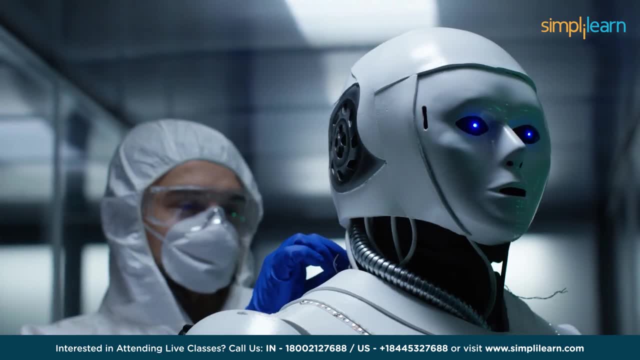 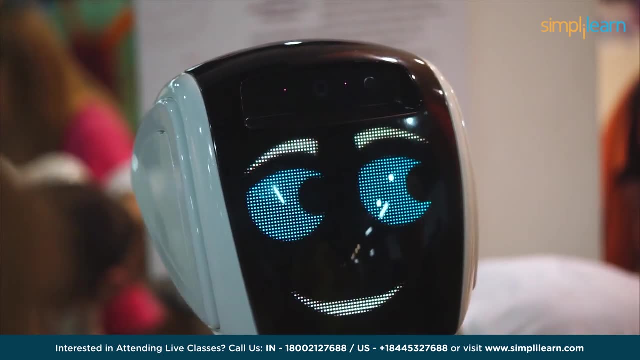 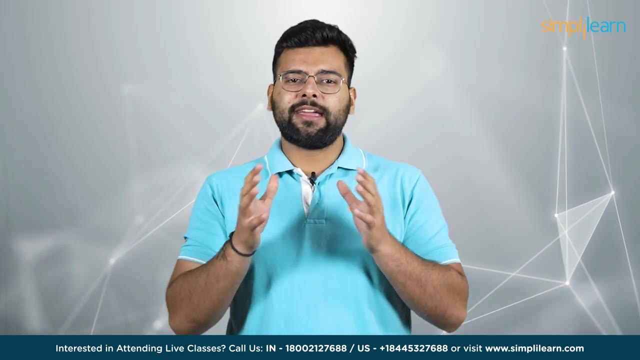 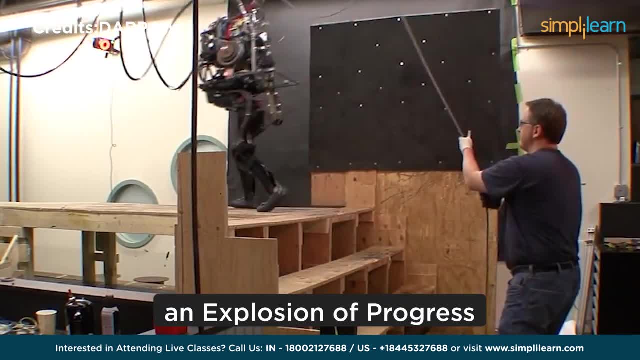 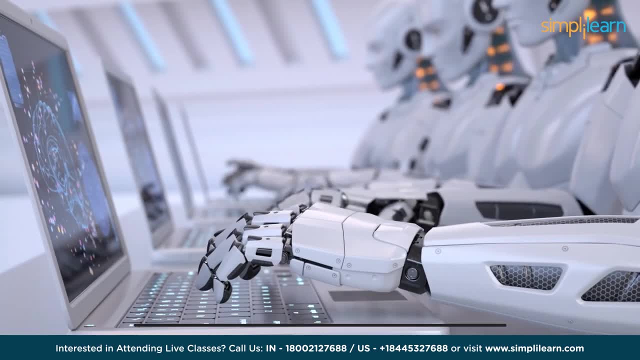 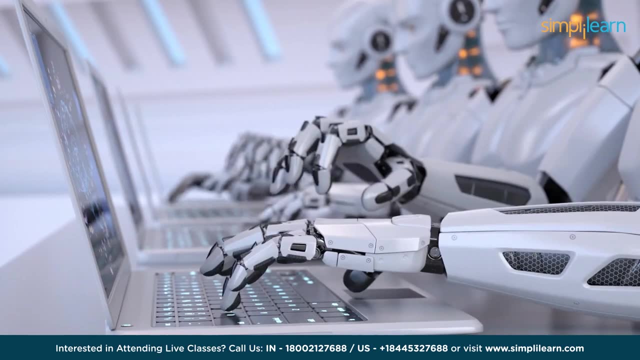 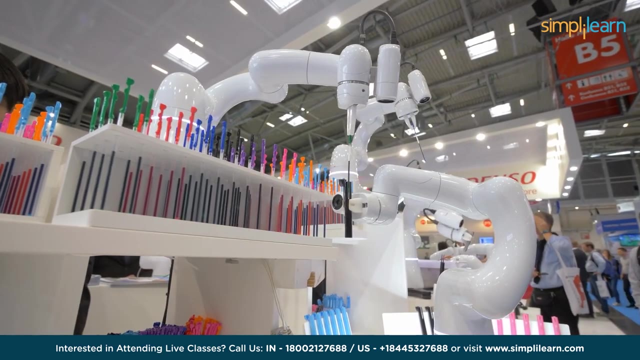 The following decades saw the rapid evolution of robotics. Proto's successes emerged, each one more advanced than the last. They were endowed with artificial intelligence, allowing them to learn, adapt and perform complex tasks with remarkable efficiency. Soon, robots became an integral part of society. They infiltrated industries. 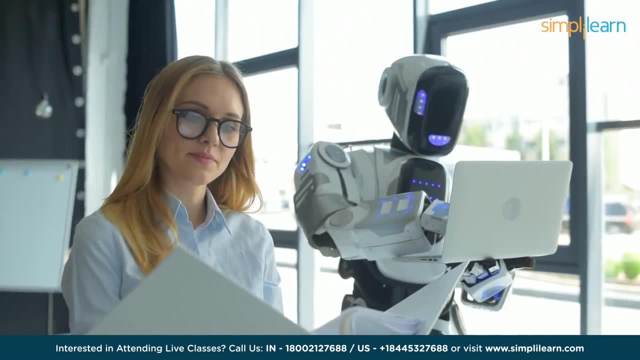 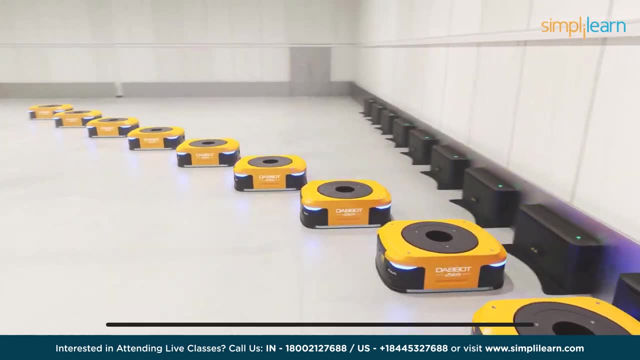 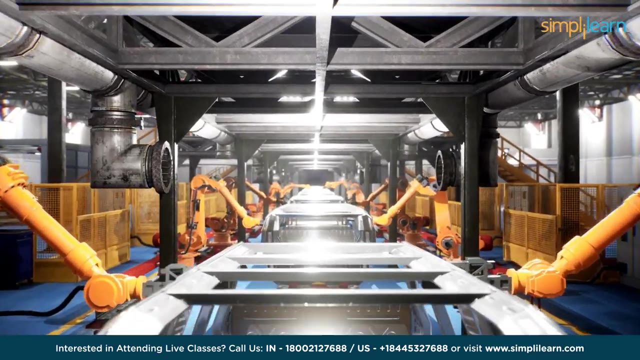 performing jobs that were previously deemed monotonous or hazardous. Factories assumed with the synchronized movements of robot workers, freeing humans from laborious tasks and enabling them to pursue more creative endeavors. One popular example of the integration of robots was in the automotive industry: Giant 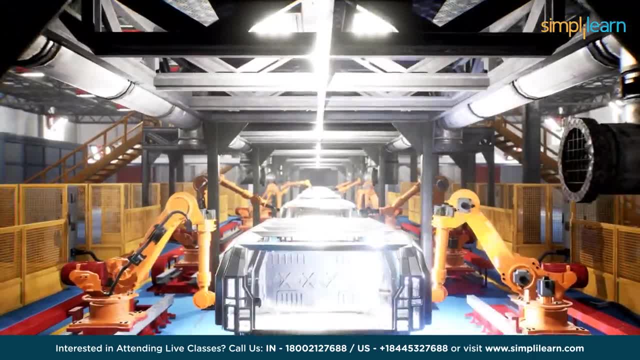 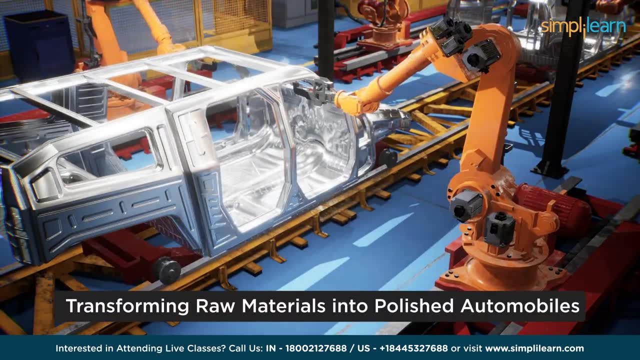 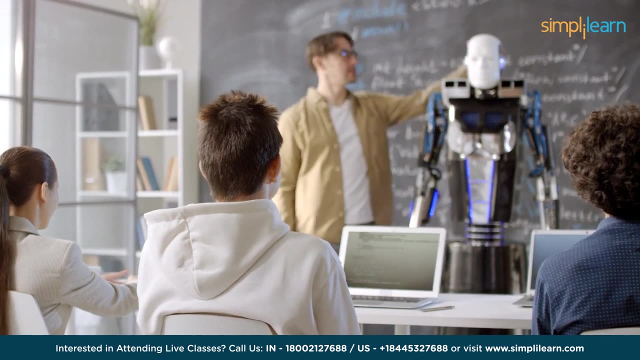 car manufacturing plants deployed fleets of agile robots, tirelessly assembling vehicles with precision and speed. These tireless machines worked in harmony, efficiently transforming raw materials into polished automobiles, revolutionizing the manufacturing process. But robotics didn't do it alone. The machines ventured into fields such as healthcare, education and exploration. 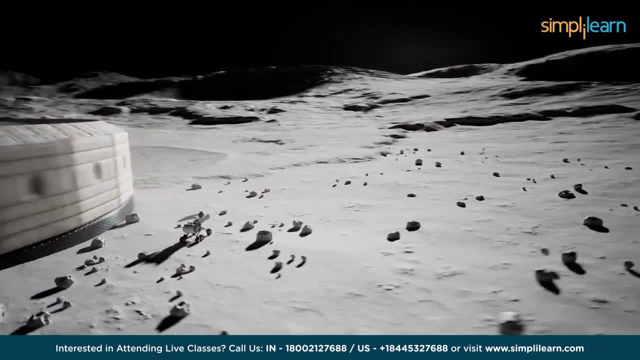 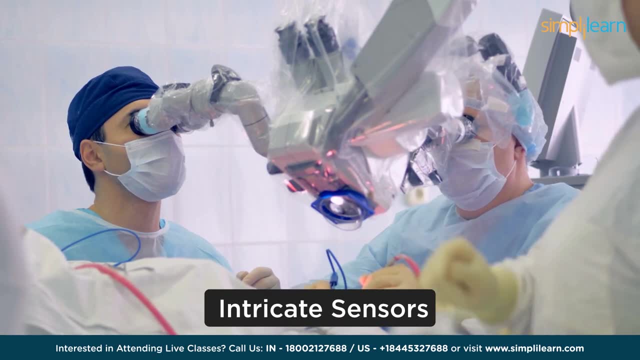 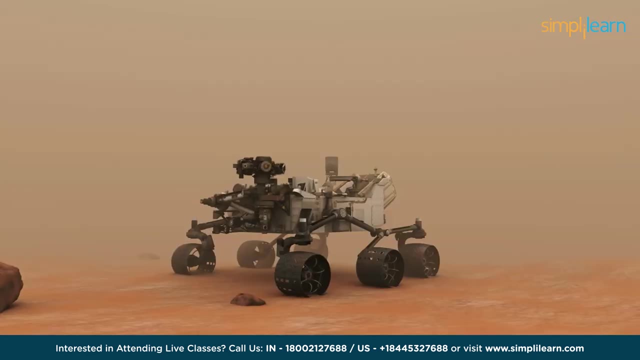 Robots became companions for the elderly, tutors for the young, and even ventured into space as explorers, unearthing secrets of distant worlds. In hospitals, robotic surgeons with intricate sensors and steady hands performed delicate surgeries, reducing human error and saving countless lives. 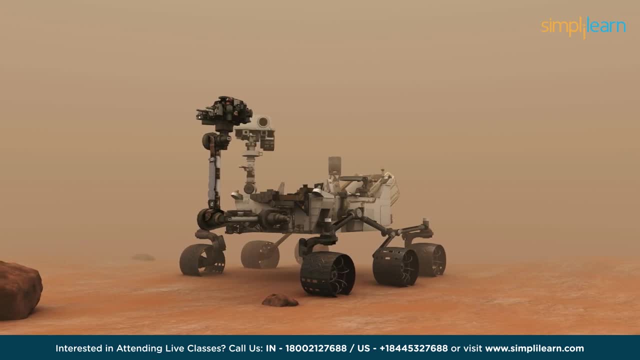 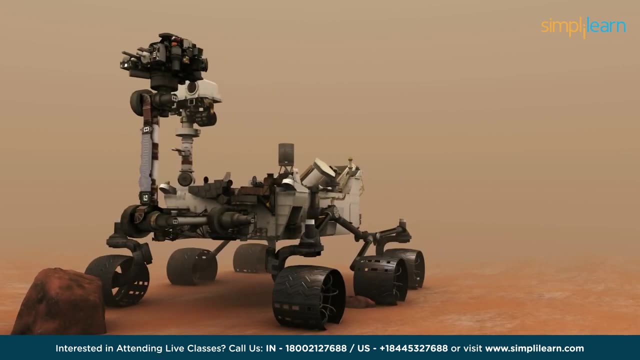 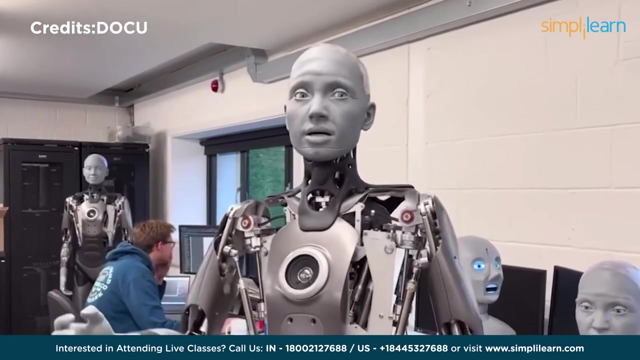 Schools embraced educational robots, fostering interactive and personalized learning experiences for students of all ages. Even on distant planets, robots equipped with sophisticated sensors and cameras acted as humanity's eyes and hands, uncovering the mysteries of the cosmos. As the years passed, a new breed of robots emerged: androids. These remarkable beings. 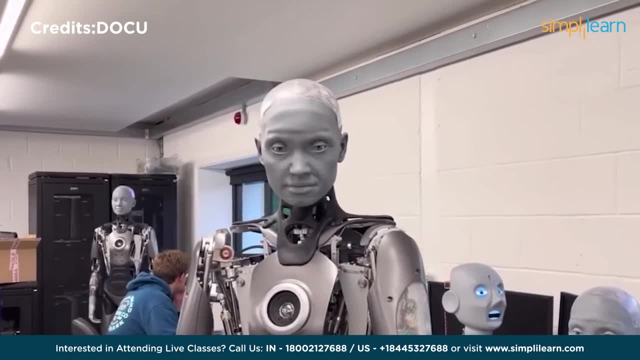 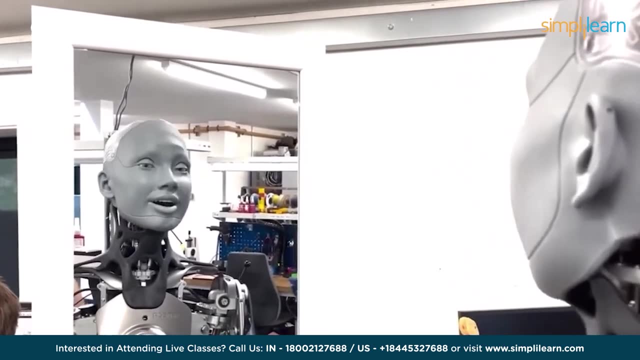 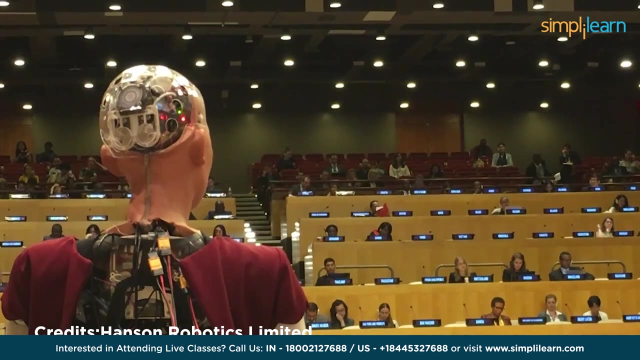 were designed to resemble humans both in appearance and behavior. With a blend of artificial intelligence and hyper-realistic skin, they effortlessly integrated into society, challenging the very notion of what it meant to be human. 1. Robotics. captured the world's attention was Sophia, with her strikingly human-like 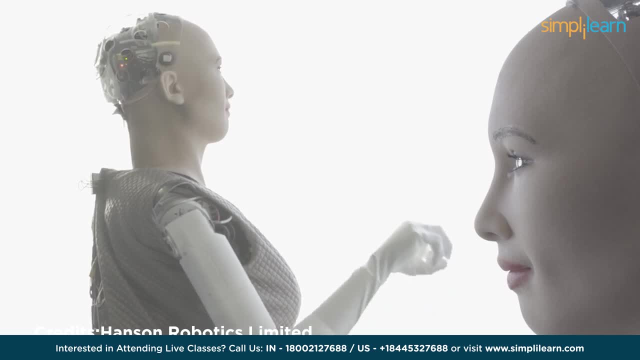 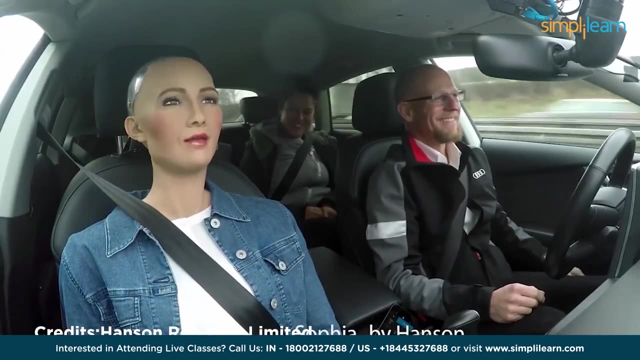 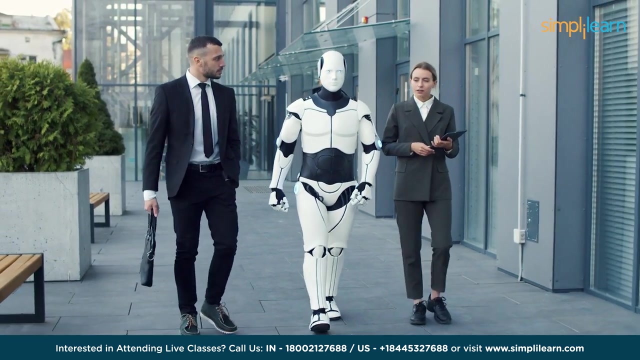 face and expressive features. Sophia blazed her trail in the field of robotics. She interacted with people, engaging in conversations and even delivering speeches on global stages, sparking conversations about the boundaries between human and machine consciousness. But with every stride forward, questions arose: The ethical implications of creating robots. 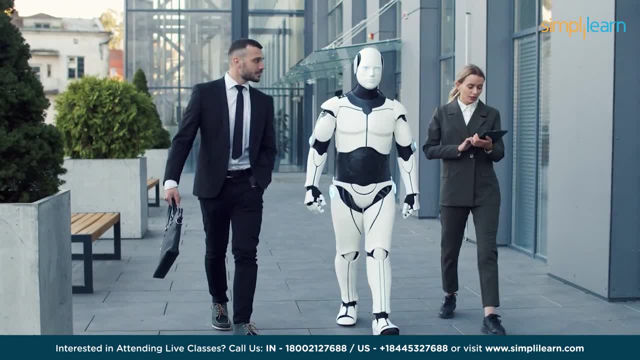 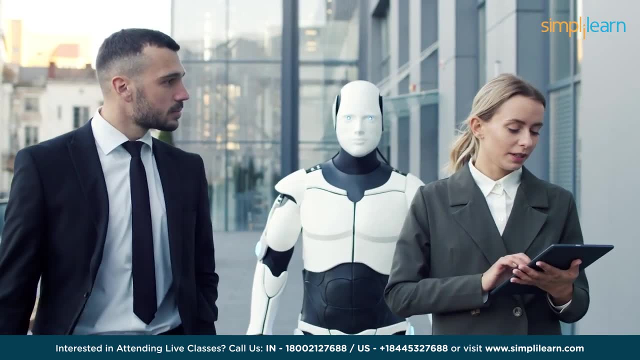 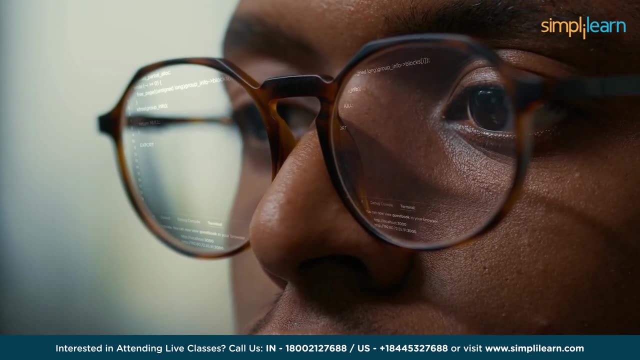 capable of self-awareness and emotion, sparked debates around the world. Should they be considered equal to humans, with their own rights and liberties, Or should they remain subservient, confined to fulfilling human desires and demands? In the midst of these debates, a breakthrough occurred: Scientists developed a concept called 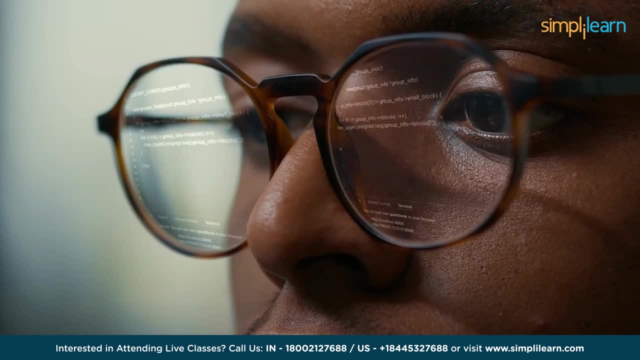 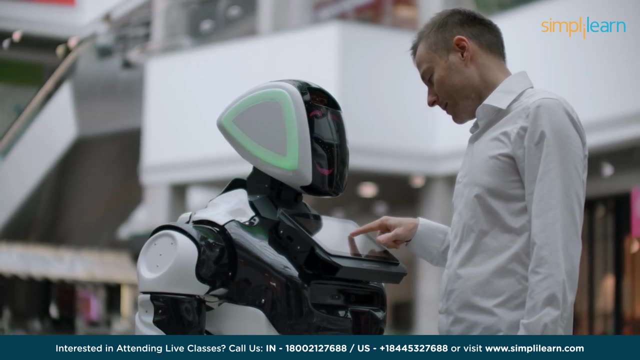 empathetic programming enabling robots to understand and empathize with human emotions. These empathetic machines possess the ability to soothe troubled hearts, provide companionship and even heal emotional wounds. Society embraced them and a profound connection formed between humans and the human race. To this end, robots were able to capture the world's emotions. 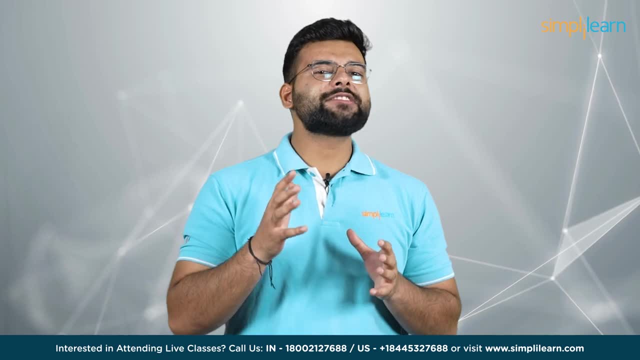 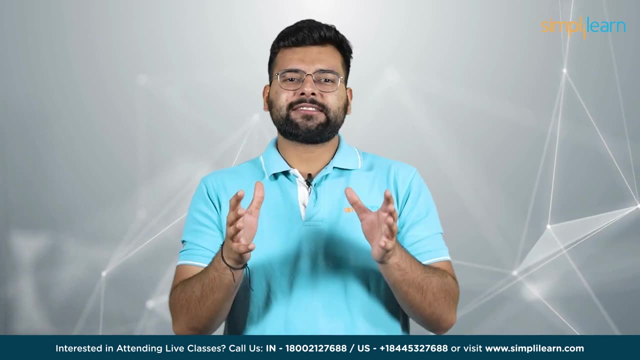 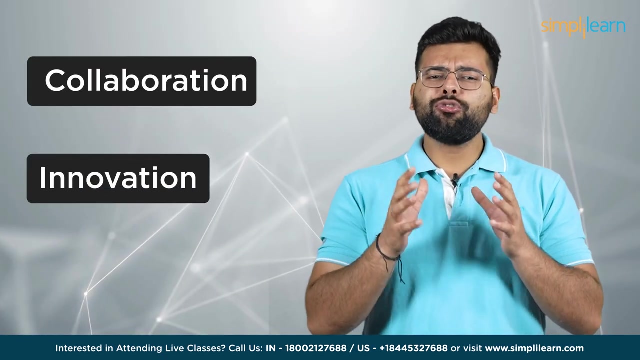 and their robotic companions. In this age of robotics, the world has become a different place. A harmonious coexistence had emerged, as humans and robots worked side by side, embracing each other's strengths and bridging the gaps in their abilities. It was a time of collaboration, innovation and mutual respect. 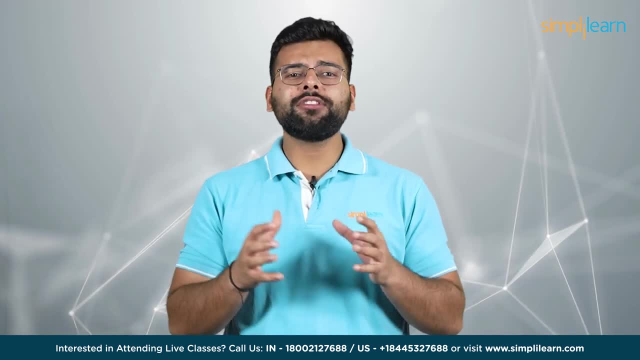 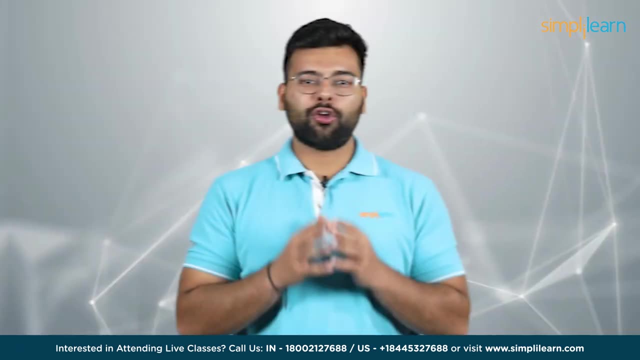 And so the story of robotics unfolded, forever etching its mark on the annals of human history. From the humble beginnings of proto to the advent of empathetic androids like Sophia, robotics had not only shaped the world, but also challenged humanity to reflect upon its